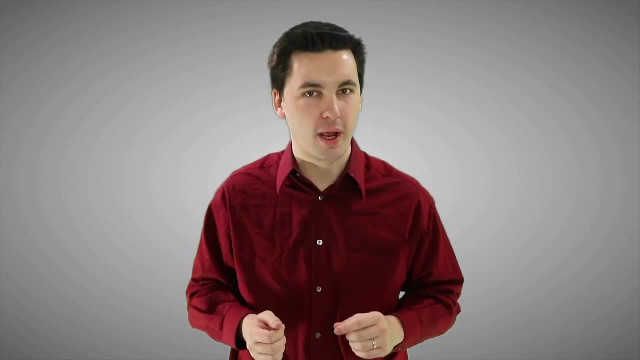 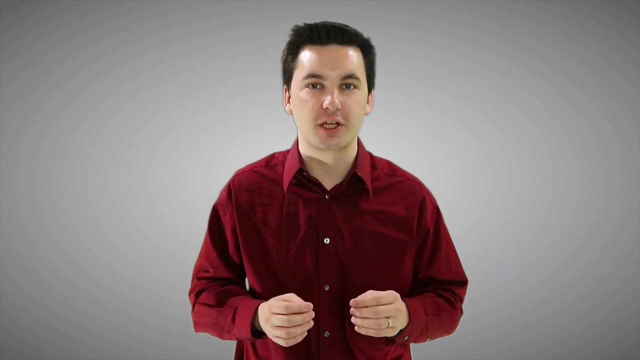 transportation. Over time, transportation's come a long way for society and we can see how that's reshaped the very cities we live in. Public transportation has made it easier for people to get around downtown and, thanks to advancements in cars and robust interstate systems, it's 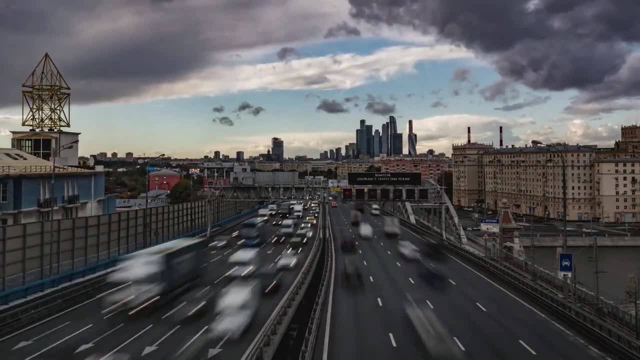 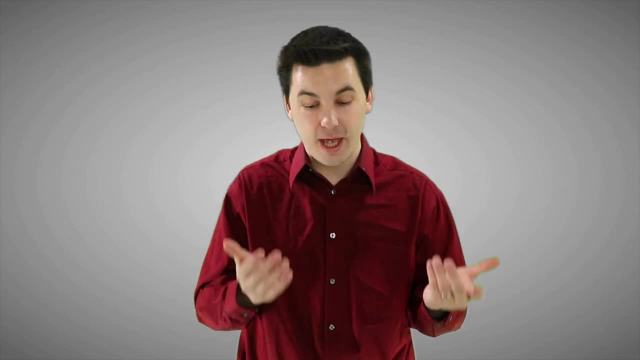 now possible for people to live in less densely populated areas in the suburbs but still have access to all the benefits that cities offer. We could also talk about advancements in communication to see how that's reshaped urban life as well- The landline, for example. 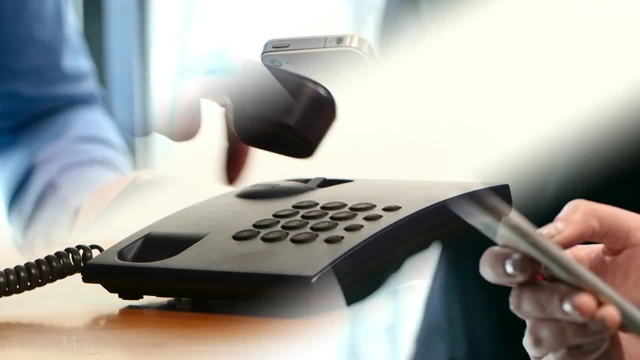 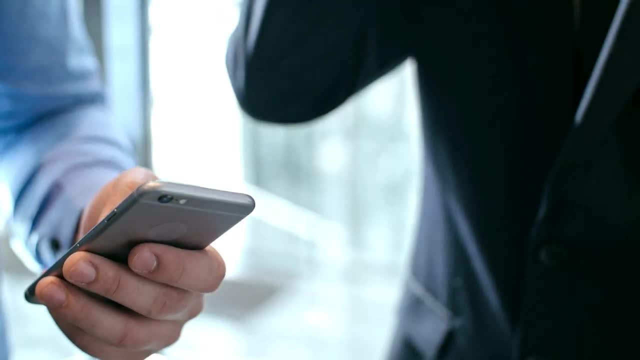 made it possible for people to connect all over the world and, with the cell phone diffusing throughout society, we now have access to the internet and soon to be, 5G, which expands where people can work and live. Today, thanks to the advancements in all of these technologies, we can have people have. 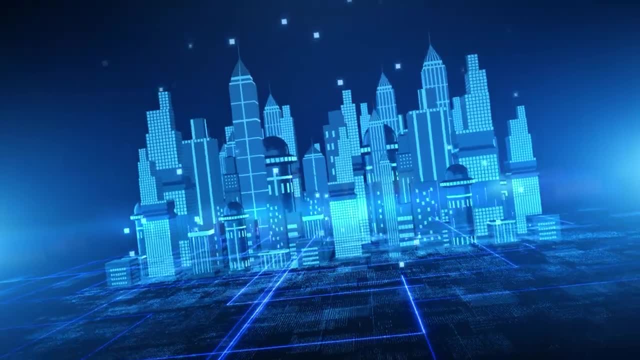 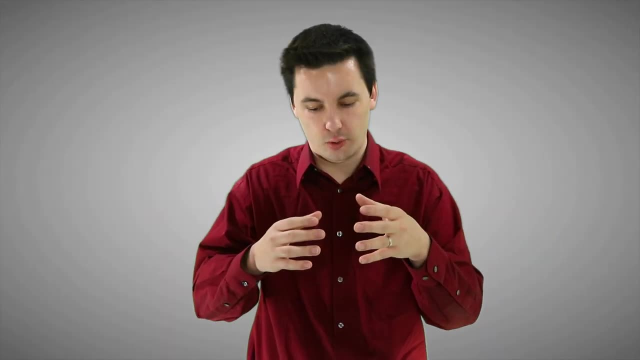 a more comfortable way of living and working from the comfort of their own living room. We can see that these advancements in communication and transportation have allowed our cities to become more connected than ever before, and not just with cities within their own region, but the nation as a whole or even a global community. Cities today interact on 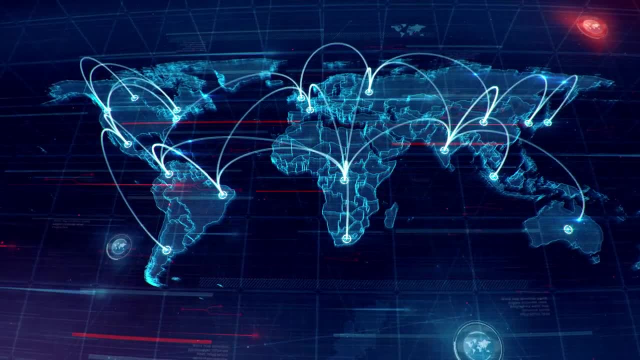 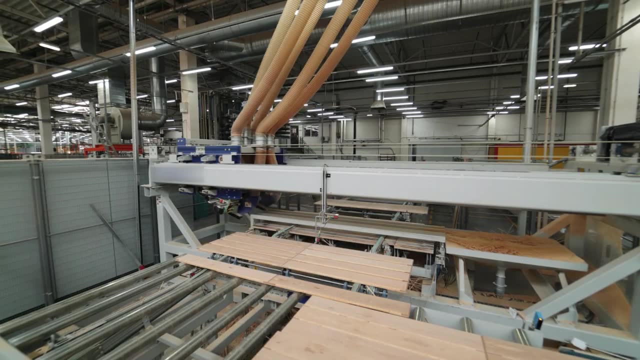 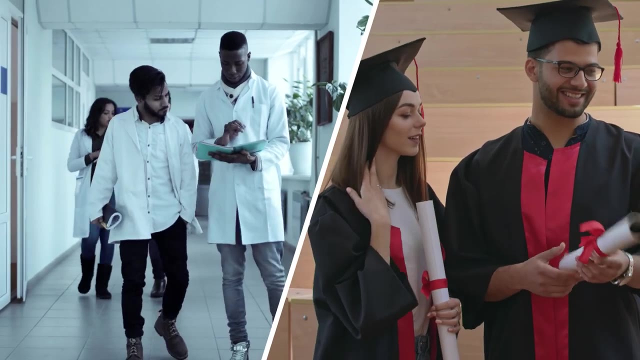 a global level, and this allows them to specialize more and it allows them to create a stronger sense of place. We can see that some cities will focus on manufacturing, while others may focus on tourism. Some will even focus on a specific industry, industry like healthcare or education. all of this creates a unique identity for a city. so today we 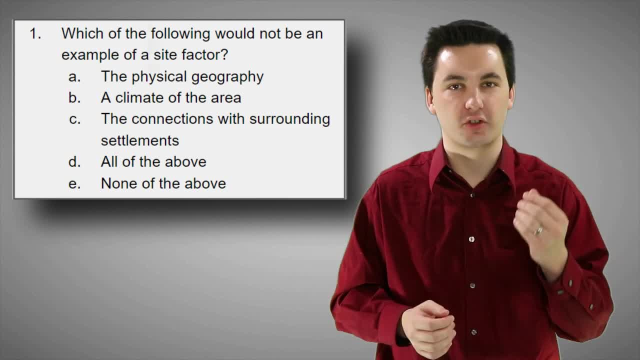 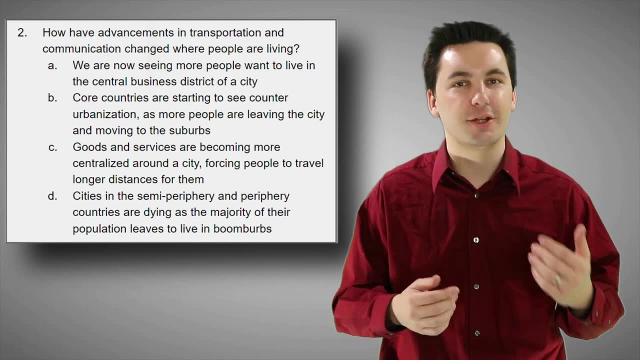 talked about different site and situation factors. we also looked at how cities are connected, transportation, communication and how all these things could impact the growth of a city. now we're going to be elaborating on these themes throughout this entire unit, but right now, what i need you to 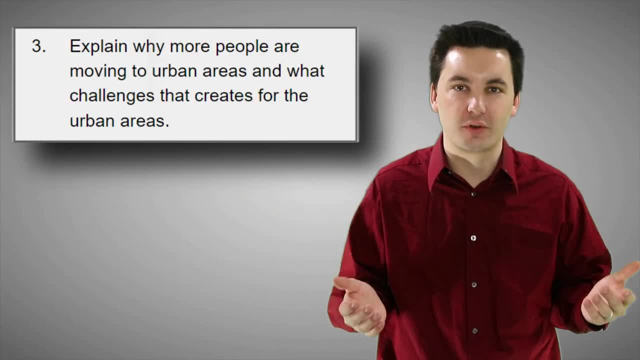 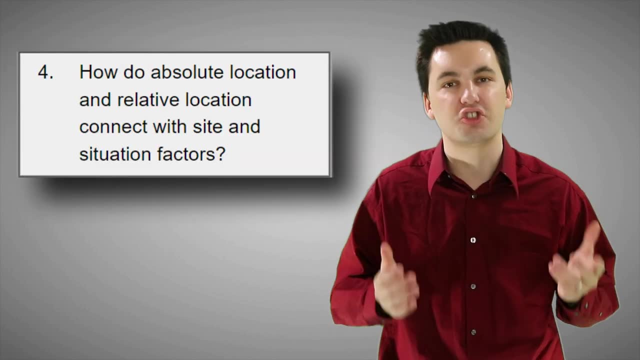 do is practice. take a second practice: the concepts we went over today. you can look at the questions on the screen and check your answers in the comments below. also, don't forget to hit that subscribe button. it's a great way to support the channel. it's free and if you change your mind, 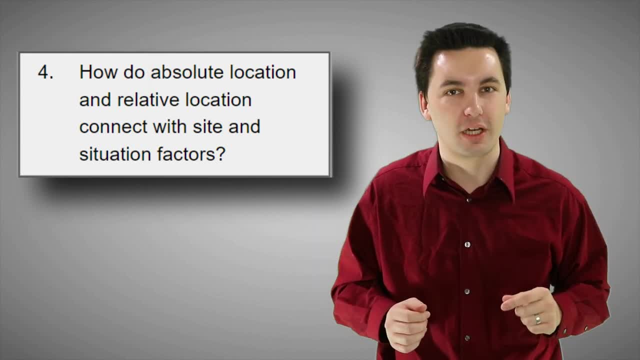 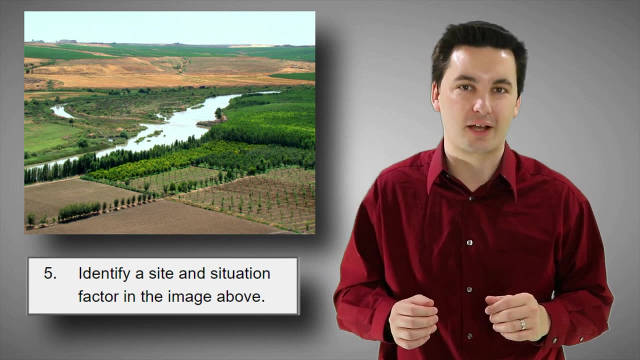 later. you can always unsubscribe, but this allows me to continue to make more videos and make sure you don't miss future videos. also, don't forget to check out the ultimate review packet if you're struggling with your ap human geography class. it's a great resource that i made to make sure that you.